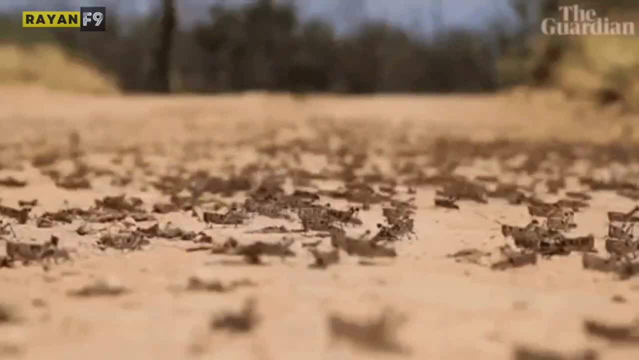 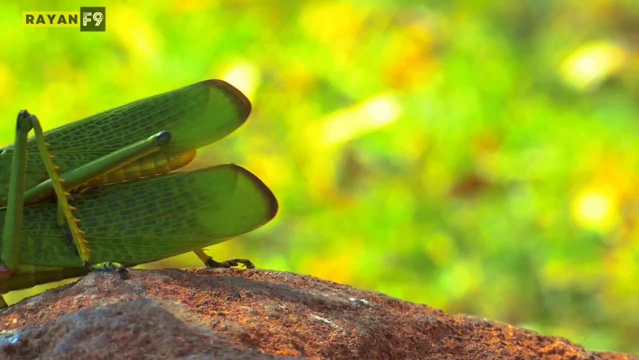 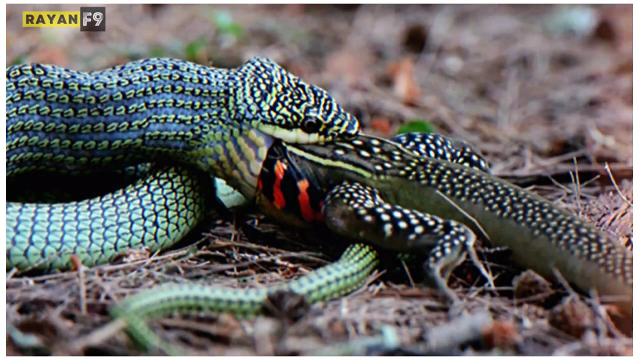 causing ripple effects throughout the food web. Number four: increased pest infestations. In the absence of snakes, the natural control of pest populations would falter. Insects such as spiders and certain types of insects that are preyed upon by snakes would proliferate. 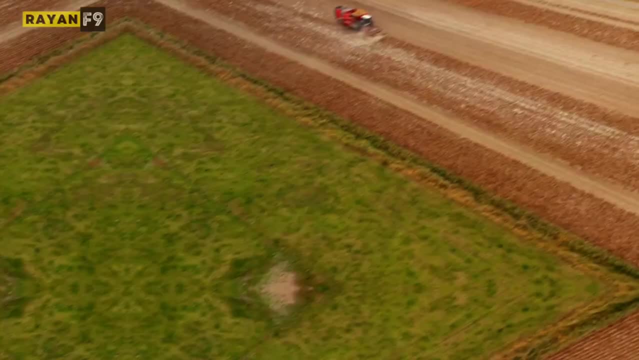 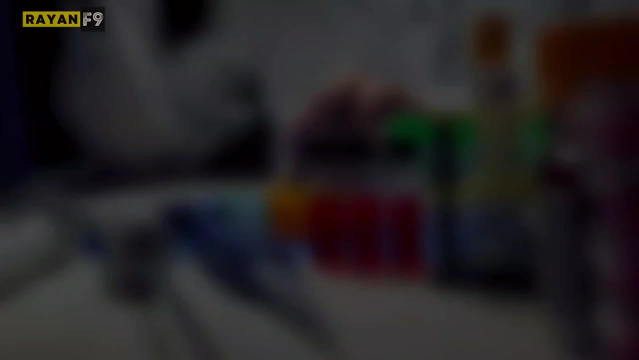 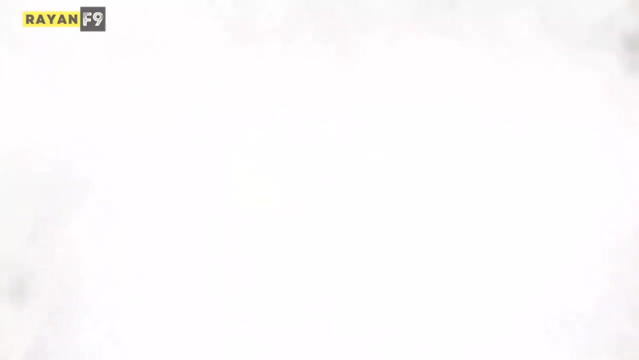 This would lead to a surge in pest infestations, affecting agriculture, public health and the overall balance of ecosystems. Number five: loss of medicinal and scientific opportunities. Snakes have long been recognized for their unique venomous properties, which have proven invaluable in the development of life-saving medicines. 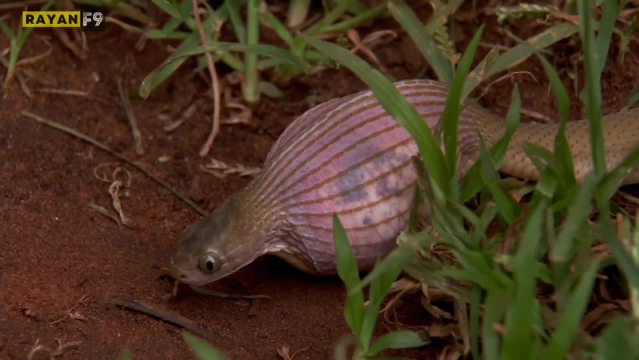 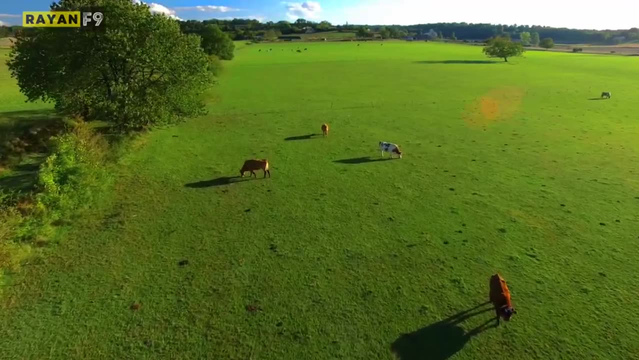 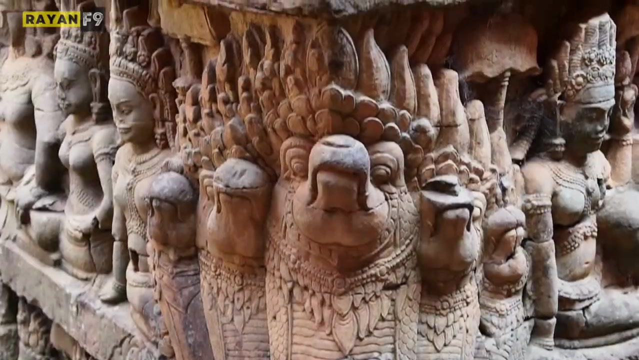 With their disappearance, potential advancements in medical treatments and scientific discoveries could be delayed or even lost entirely. Number six: social and cultural impact. The snakes have long been a subject of fascination and fear in human culture. From ancient myths and legends to modern movies and literature, snakes have left an indelible mark on our 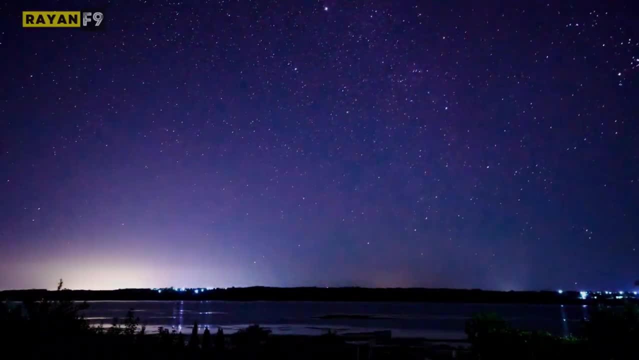 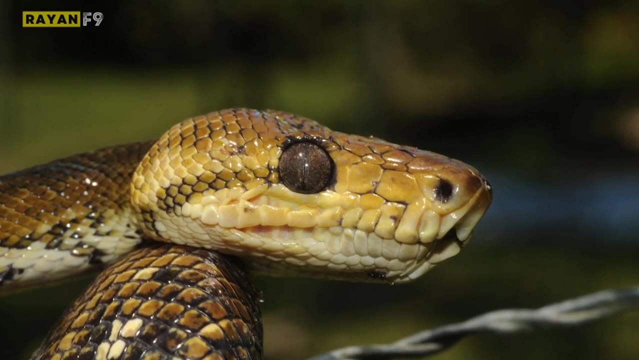 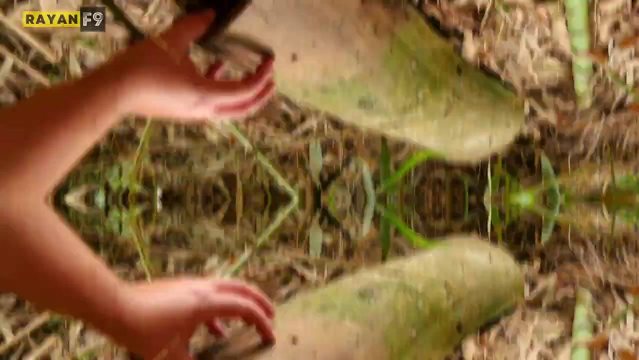 collective imagination. The absence of snakes would significantly impact cultural practices, traditional beliefs and even tourism centered around snake-related attractions. Number seven: environmental repercussions. Beyond the immediate effects, the absence of snakes could lead to long-term environmental repercussions, The disruption of ecosystems and the loss 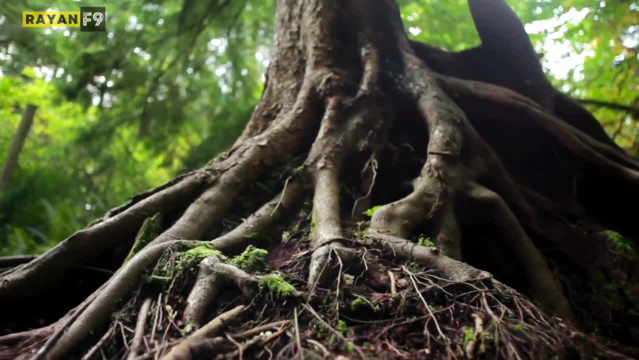 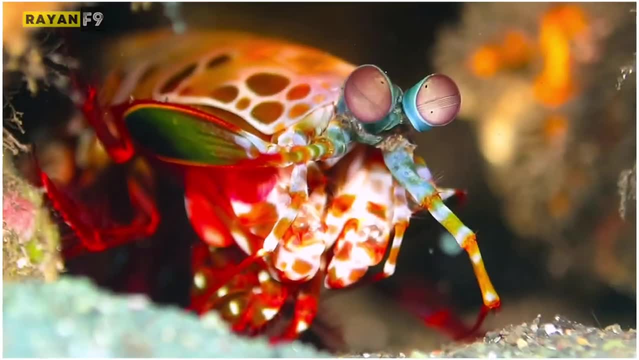 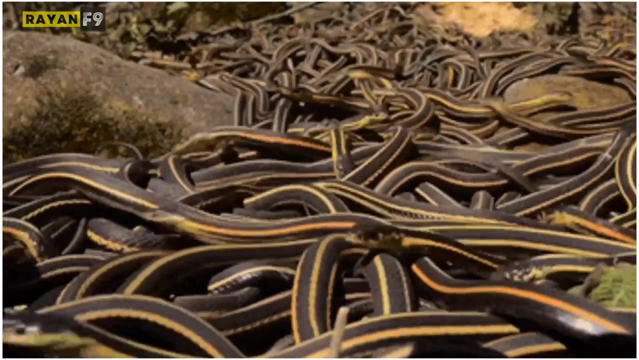 of key species can have cascading effects, potentially threatening the survival of other plants and animals, further destabilizing the delicate balance of our planet's biodiversity. Conclusion: As we conclude our journey into a world without snakes for a year, it becomes evident that their disappearance would have profound consequences. 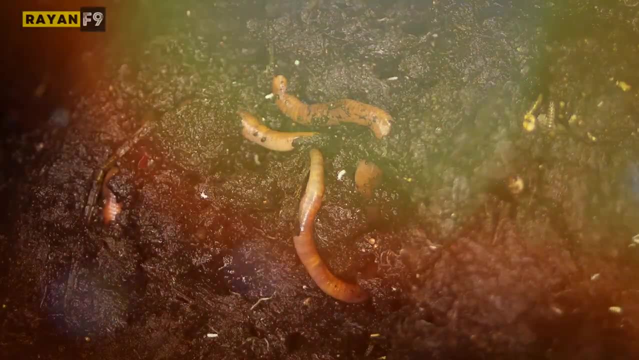 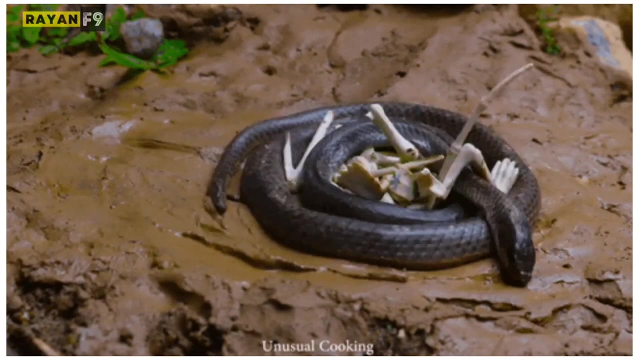 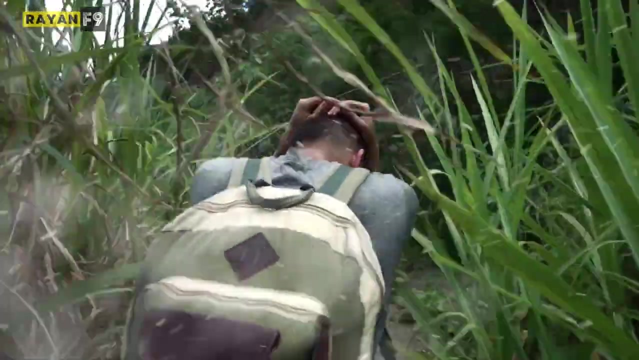 from ecological imbalances and agricultural problems. Number seven: The lack of natural and agricultural challenges to cultural and scientific setbacks. The absence of these enigmatic creatures would leave a significant void in our natural world. So depreciate and value the critical role snakes play in maintaining the delicate harmony of our planet's ecosystems. 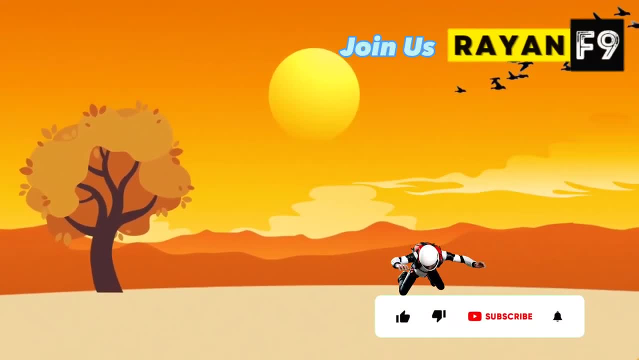 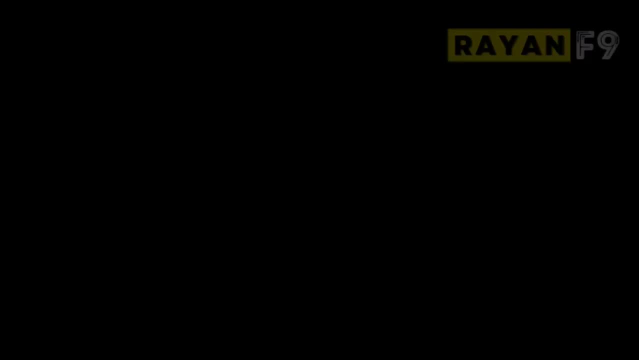 Thank you for joining us today. Don't forget to like, comment and subscribe to our channel for more captivating explorations of the natural world. Until next time, stay curious and keep exploring.